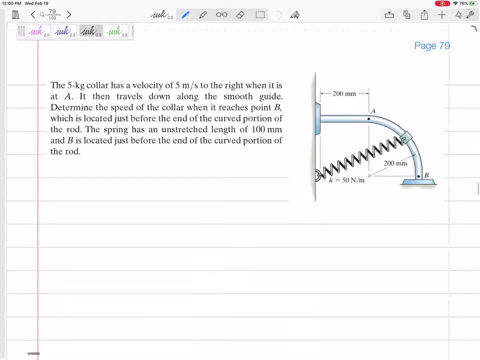 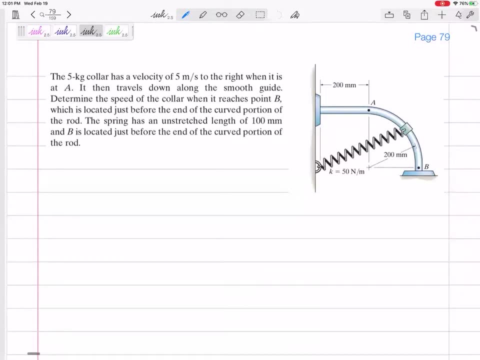 Alright, So let's look at this problem in our notes and let's organize our thoughts with conservation of energy. And I mean, obviously we're going to do that because we're in this section, but why might we use conservation of energy? 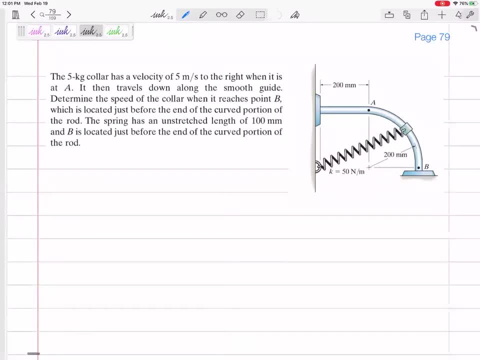 in problems where you have an object, that's kind of going from one initial point to one final point and you're given or you want to know the velocity, which is what we have here. Five kilogram collar has an initial velocity of five meters per second when it's at A. 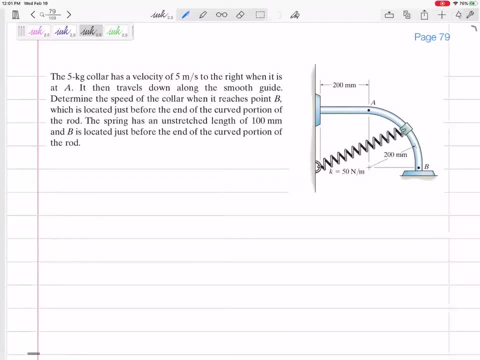 and then travels along the smooth guide to determine the speed of the collar when it reaches point B. Alright, so make sure, For all of these problems that we're doing, that you can visualize where is it starting, where is it ending, right? 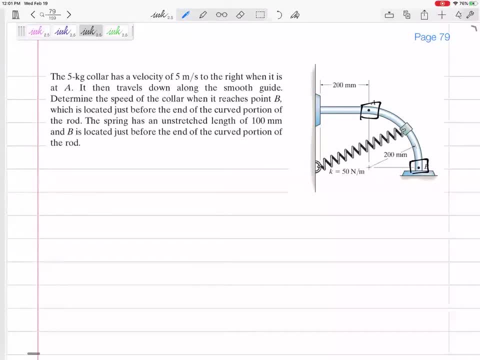 So this one starts at A and then it goes to B. Okay, so the point B is located just before the end of the curved portion. Spring has to unchange like 100 millimeters. And again B is located just before the end of the curved portion of the rod. 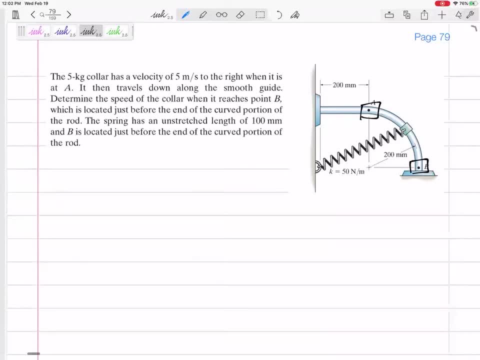 All of these problems. like point B, it hasn't hit the wall yet. all right, We haven't done problems where we're trying to find something after it hits the ground or hits the wall. So don't tell me like the final velocity there is zero. 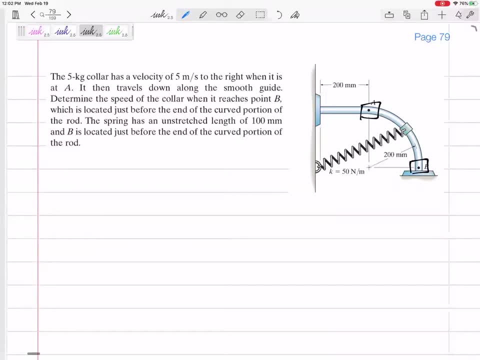 It's right before it hits the wall at B. So let's, I want to organize our thoughts with conservation of energy potential plus kinetic plus any. this is the non-conserved work, So this isn't gravity and springs. 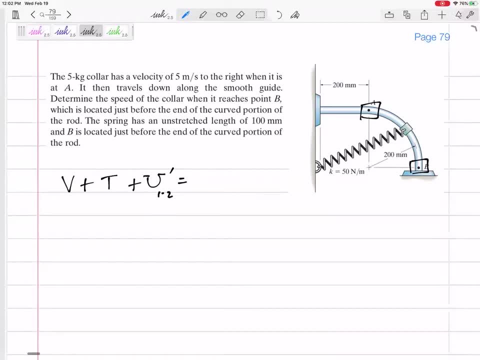 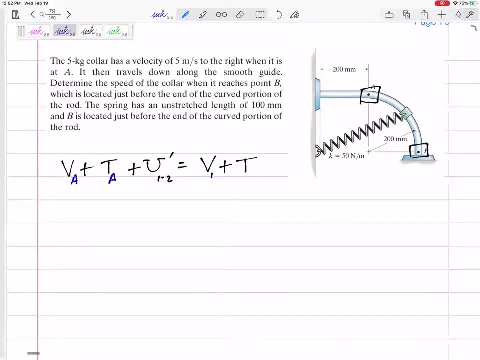 There's work like: due to a force equals the final B plus T, And so maybe we could say: all right, this is at A, this is at B, right here, All right. so this potential energy could be both gravity and spring. 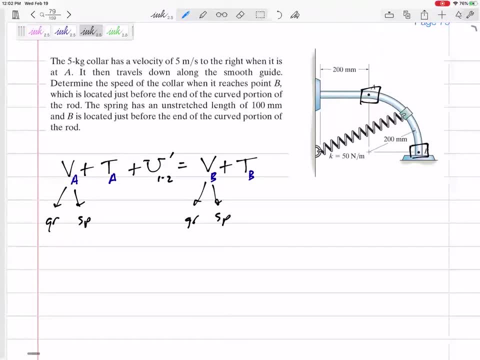 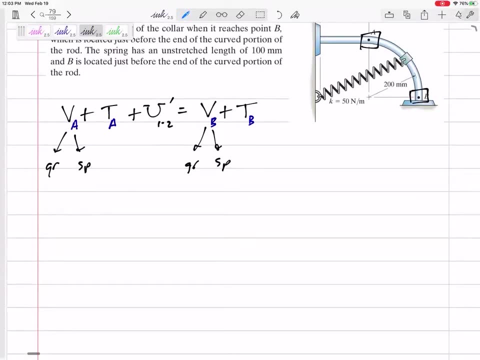 This potential energy, both gravity and spring, So don't forget both of those. Now, some of these might be zero. Maybe you could go ahead and mark them zero right now, But I like to go ahead and write out the whole: MGH plus one-half KX squared. 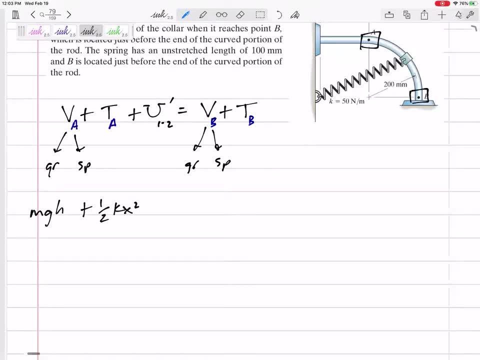 the potential energy in gravity, plus potential energy in a spring, plus the kinetic energy. one-half MV squared plus any. I'm going to put FD, but technically this is sometimes integral. FDS might be zero. It's only FD if it's a constant force and it's in the same direction. 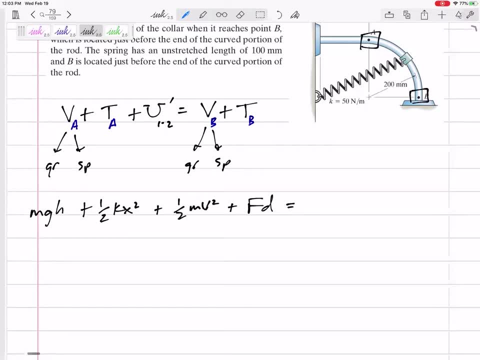 If the force is in the same direction as the displacement. So over here, this would be MGH plus one-half KX squared plus one-half MV squared. All of this on the left is the initial. All of this on the right is final. 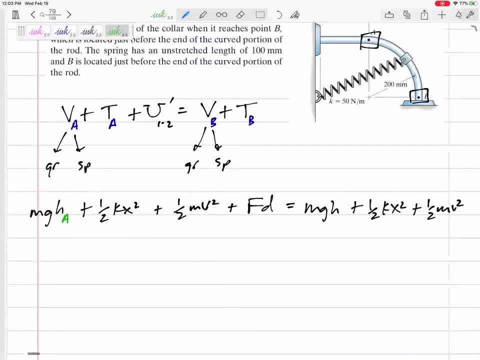 Maybe we could say the height at A, the X when it's at A, the velocity when it's at A, versus the height at B, the X when it's at B, the velocity when it's at B. Also, I like to 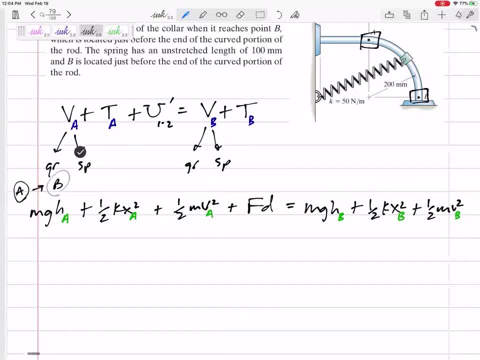 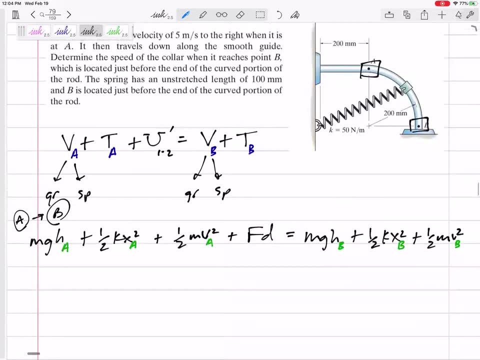 I like to sometimes write. Okay, just remind myself. All right, I'm going from A to B. This is a conservation of energy equation: from A to B, All right. so now let's think about the potential energy in height, potential energy in the spring. 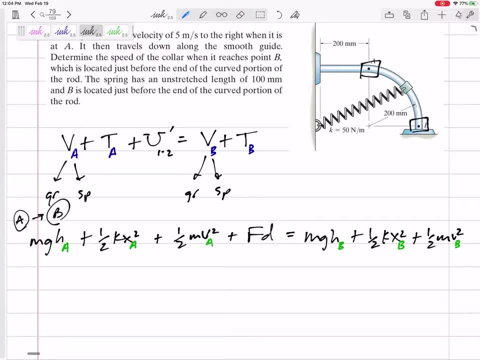 Let's think about all these terms. right, I like to write that whole equation and now I can break it up into bite-sized pieces. Okay, so, MGH, MGH, you have to choose up to be positive, but you can set your ground to be wherever you want it to be. 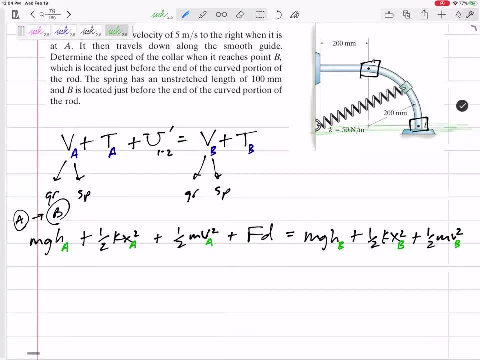 How about I'm going to do this? I'm going to set- That's going to be my ground, which would make that height zero, and it would make this height when it's at A See, if that has a radius of 200. 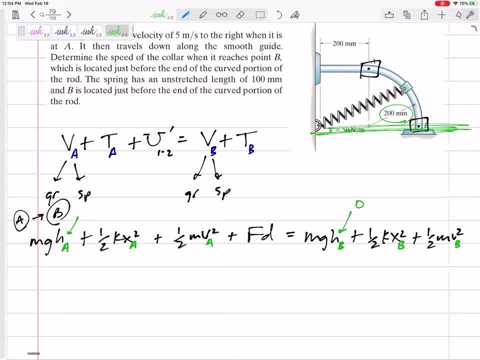 It would be 200 right there. Should we put 200? 200.. I think I'm going to put 0.2, just because I know that G is 9.81 meters per second. The velocity is Or meters per second squared. 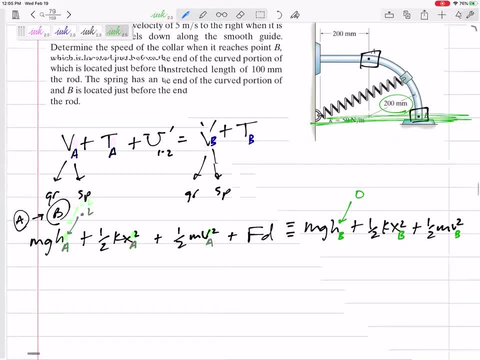 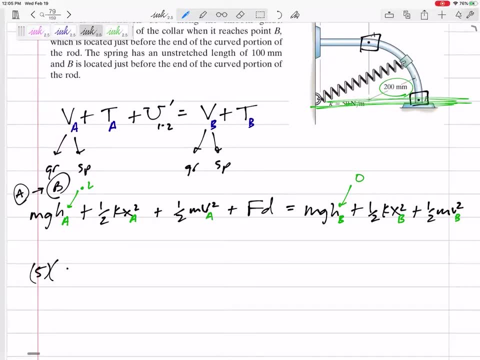 Velocity is in meters per second, So let's do 0.2, keep everything in meters, All right. the mass: a 5-kilogram collar. the G: 9.81,. the height: 0.2 meters. 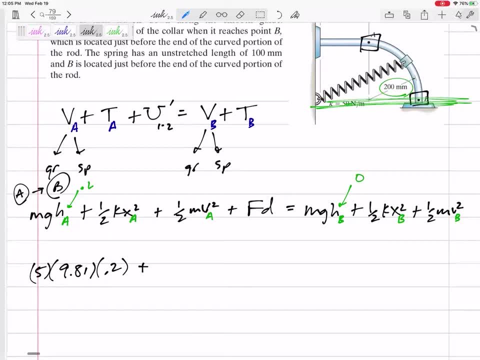 Probably should write my units in there. but units do work out. And remember we're not going to put in negative 9.81.. That's good. It's not acceleration, It's just G, Just MGH. just plug in the magnitude of G. 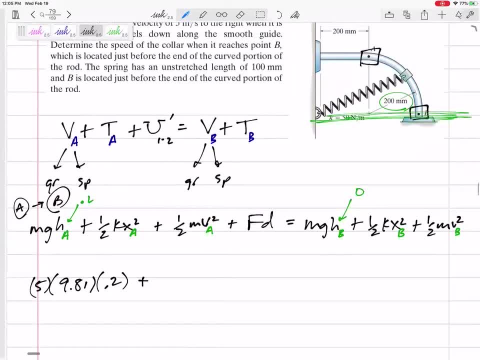 All right now. 1 half KX squared When it's at A. what is the X? What is the X? X is not the length of the spring, but the stretch of the spring. When it's at A, the spring would be that long, right, that length. 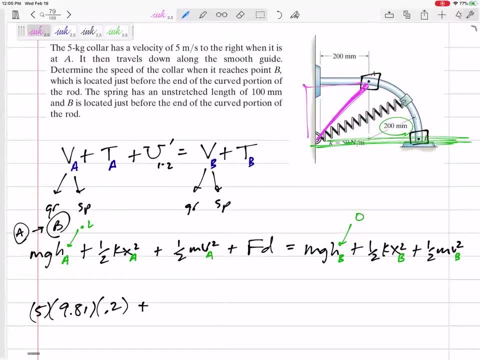 What is that length? Well, it's 200 by 200.. 200 rectangle the hypotenuse, So 200 squared plus 200 squared, This length 287.8 millimeters. All right, that's the length of the spring. 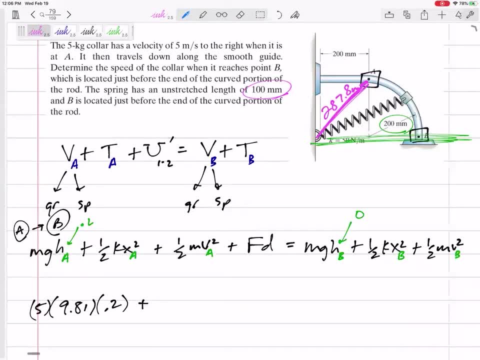 But what is the stretch? Well, if it's unstretched at 100 and now it's at 287, its X is 187.8.. I think I'm going to change that to meters. So let's say the 1 half K. 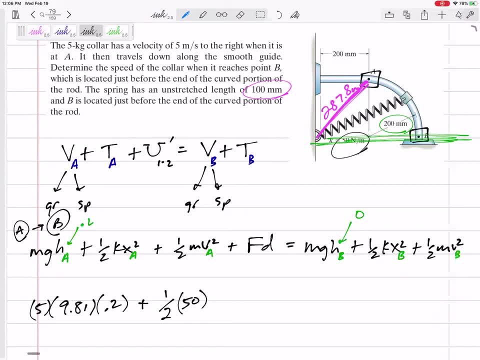 And here's really why I need to change it to meters, because that's 50 newtons per meter And the X would be point. So let's say 187.8 millimeters, or 0.1878 meters squared- Don't forget to square these things. 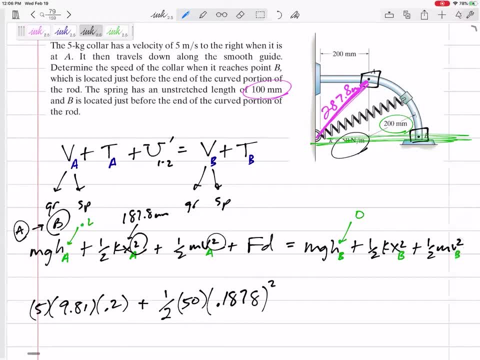 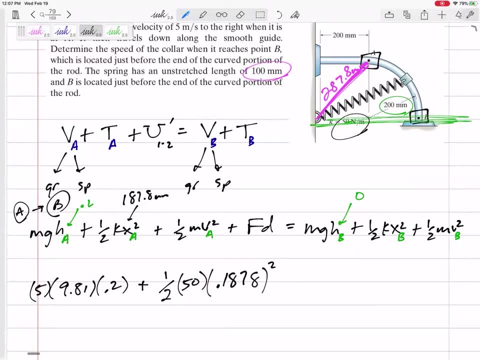 And obviously don't square the MGH. That's a common mistake- is not squaring either the X squared or the B squared. And if I kept it up with my units, that might alert me to: hey, my units don't quite work out. 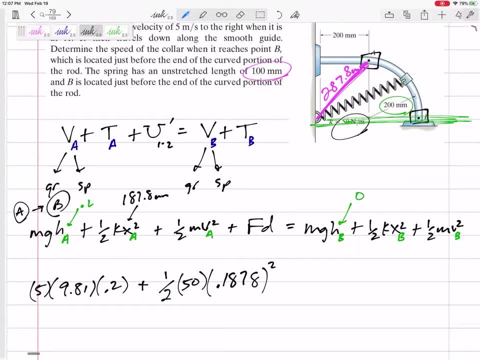 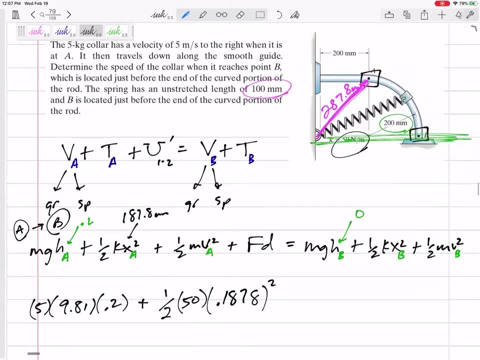 I need to square that. All right Now. the 1 half MV squared. initial. Did it say it started from rest? Some of these say it starts from rest, so don't have to worry about that, But this one it did not say started from rest. 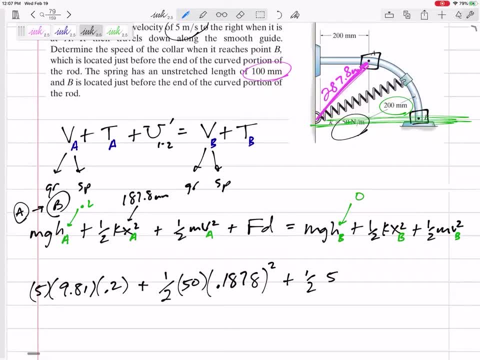 It has velocity of 5.. 1 half MV squared right there, All right. This FD is. is there any force drawn on here? Is there any force that does work besides gravity, besides spring? We already took care of those. Is there a rope that is pulling it some distance? 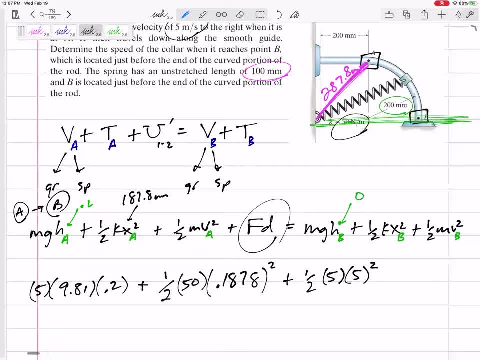 No, No, I mean the only other forces. here there's a normal force of the rod on the collar, But those never do any work. So I'd say this problem has no FD. External: no non-conserved work term equals the final MGH. 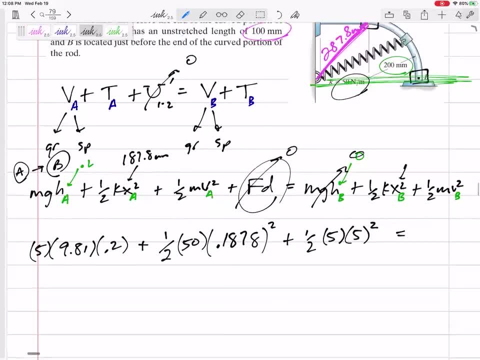 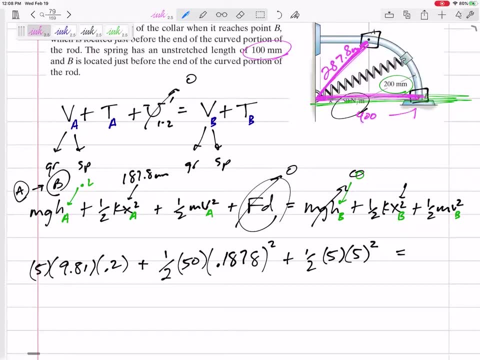 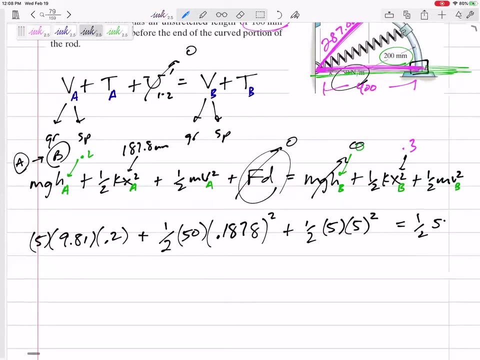 Well, it ends at zero. It ends. what would this X be? Well, this length would be 400.. And its unstretched length is 100, so 0.3.. 1 half K, 0.3 squared. 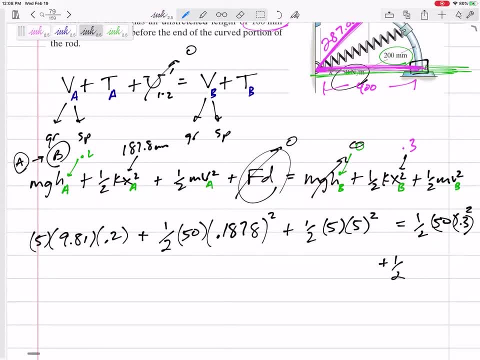 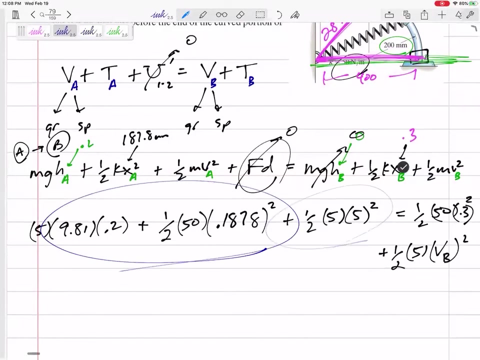 All right there, Plus 1 half MV is what we're looking for. 1 half MV is what we're looking for. Not too bad. Not too bad. I mean, this is conservation of energy: The initial potential energy plus the initial kinetic energy. 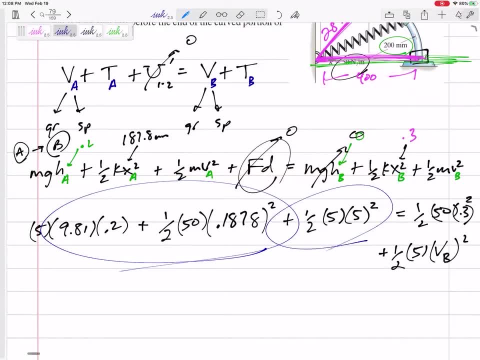 Now it's just changed, It's just transferred. Some of that potential Potential energy becomes kinetic energy and we're left with that energy. right there, It's only one equation, right, This energy is only one equation. It's not an X equation or a Y equation. 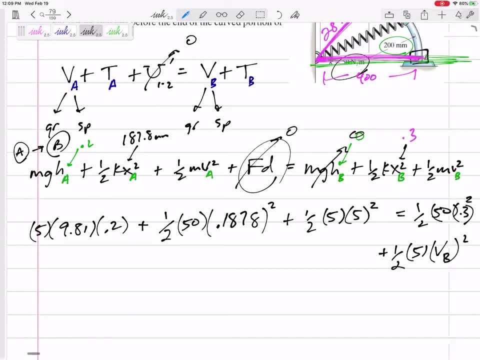 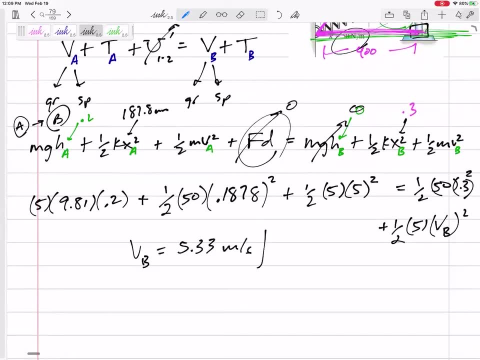 It's a magnitude, And so we can only solve for one unknown, and we're golden right. We have one unknown VB Velocity of B 5.33 meters per second Box. that, in This one, actually doesn't tell me the direction of that. 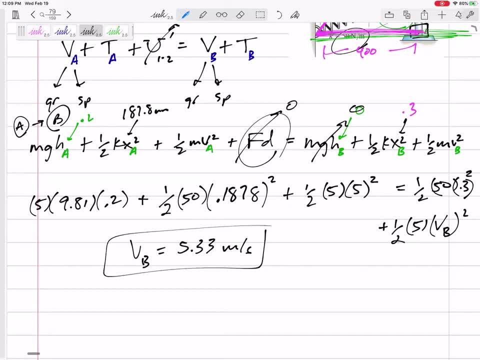 It could be plus or minus, It could be left right up down at some angle. That's the speed. And if we ever wanted to figure out the, you know, we know the direction, But this equation doesn't give us directions. 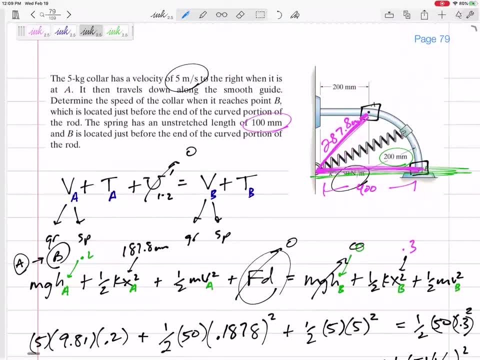 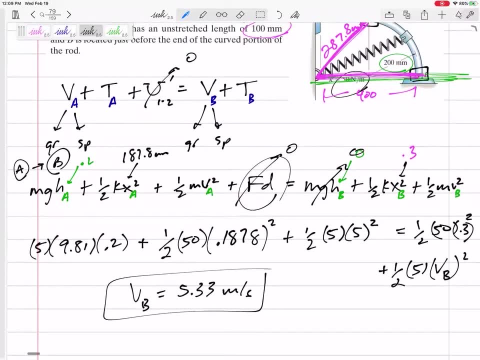 Okay, now let me add this: This one doesn't ask and don't answer questions. I'm not asking, But another common thing for me to ask is: hey, what's the normal force of the rod on the collar Down there at V? 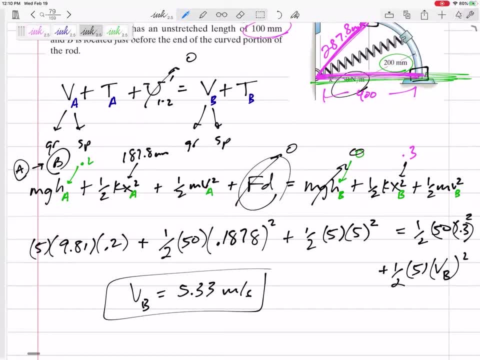 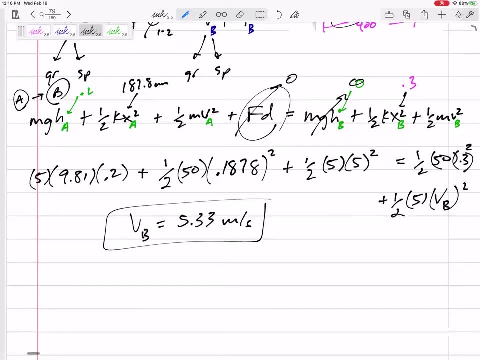 So you know, even though this is an energy problem, even though this might be, even though I tell you, hey, problem number three on the test is an energy problem, it might be energy and free body diagram, Or we'll do one that's energy and projectile. 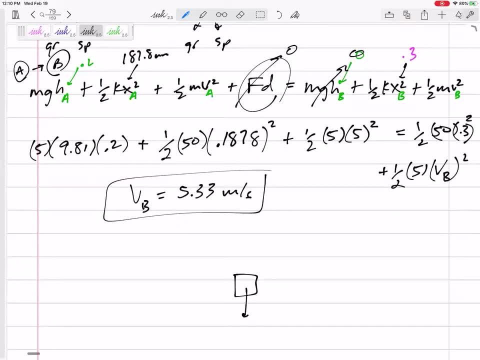 So this one, if I had asked for the normal force, we would need to draw a free body diagram. And you know, I think Solve for the normal force. Y'all know that the normal force of a rod, that's on a collar, that's on a rod. 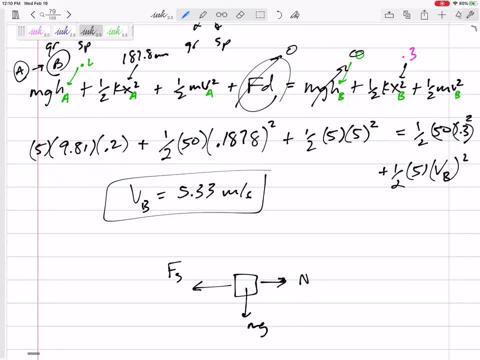 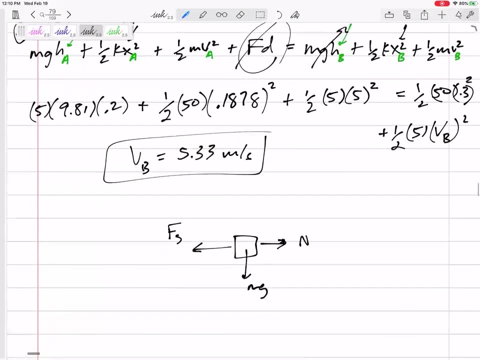 normal force between the two, you know, is perpendicular to the rod. So down here at V the normal force would be either right or left, either right or left. Draw it one way and then guess, And if it comes out negative, it was the other way. 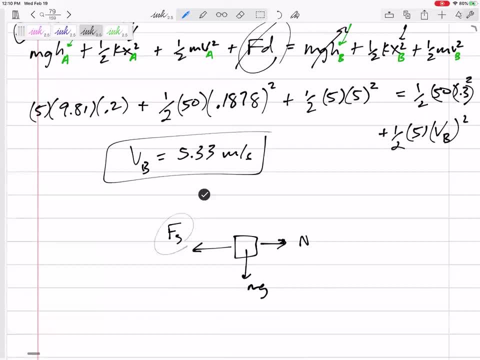 So for this one, first of all, you do need to know that the force in a spring is what we're not talking about: energy. It's not one half KX. where that's energy, That's potential energy Force, is K delta X. 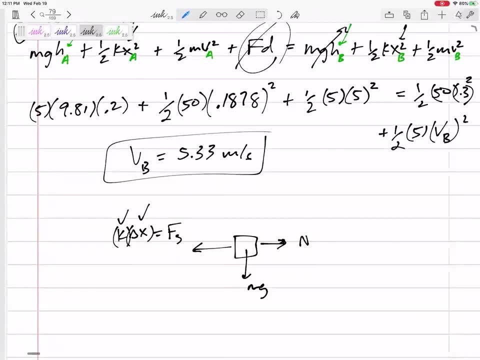 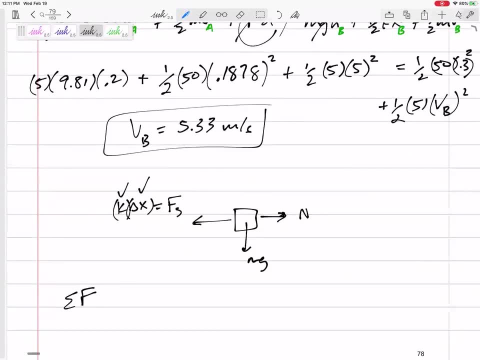 So if we, if we know the K is 50, we know the delta, X would be point three, We know that force, And so I would just sum the forces in this direction, And don't forget if it's traveling a circular path. 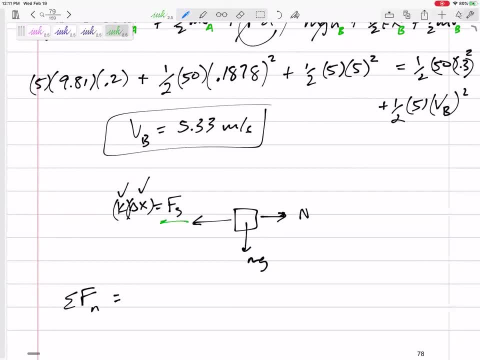 So that's, That's a normal direction. I would sum the forces, normal, tangential. So I'd sum the forces in normal negative K, delta, X plus N equals not zero, but M, V squared over row. And so now, if I know the V, I know the M, I know you know everything except for N.